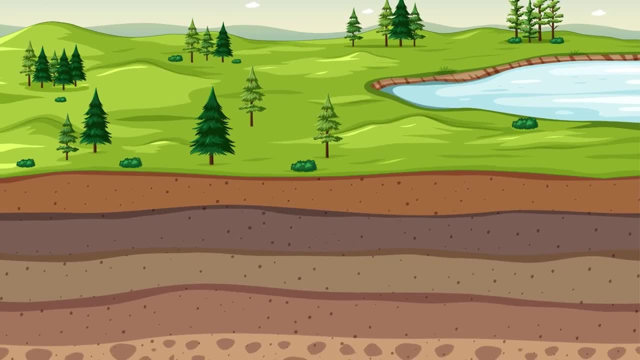 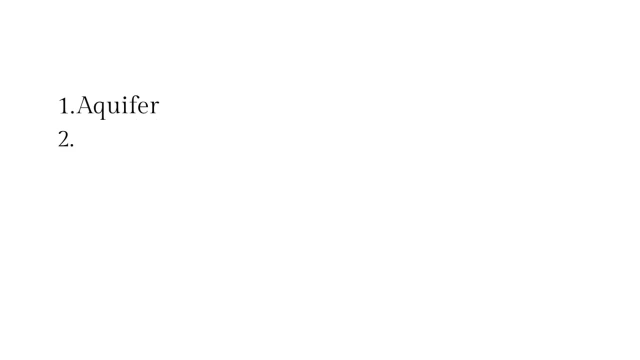 Groundwater occurs in many types of geological formations under the ground, some of which can be accessed from the surface, while some cannot. The major four types of water-bearing formations under the ground are aquifer, aquaclude, aquitard and aquifuge. We will learn about each of these geological 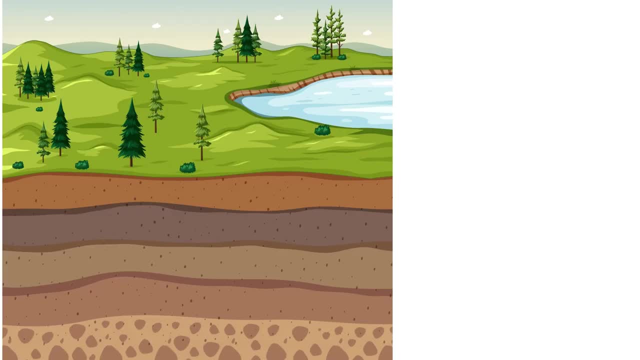 formations in detail. Let's consider a ground cross-section with the following terrain. We will assume the water table of this terrain as follows: A water table describes the boundary between water-saturated ground and unsaturated ground. Now, below the water table, there are small water pockets called geological formations. 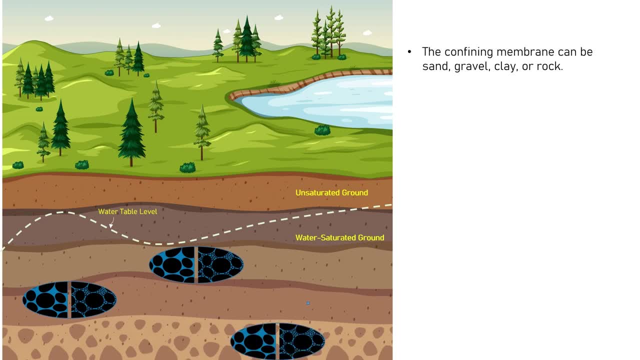 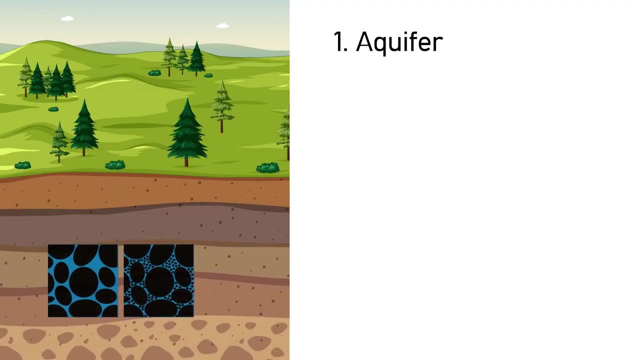 or water-bearing formations, as shown in the figure. This water is confined within gravel, sand or clay. Different confining membranes show different characteristics, Hence, based on the water movement and storage properties, these formations can be aquifer, aquitard, aquaclude or aquifuge. An aquifer is a geological formation that allows. 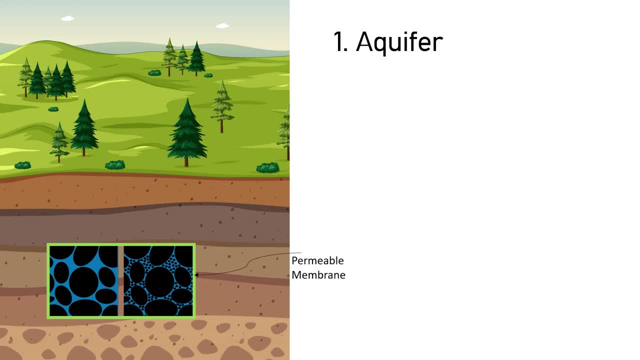 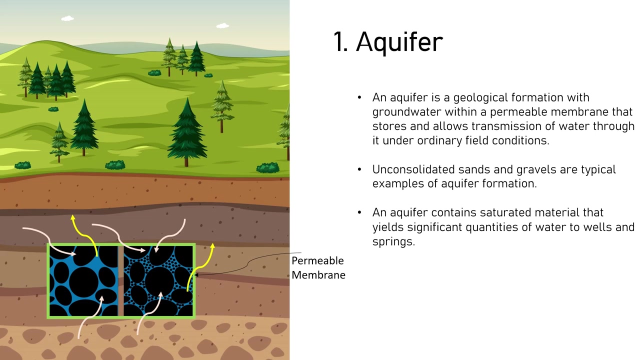 both storage and transfer of water from it. Here the groundwater is stored within a permeable membrane that stores and allows transmission of water through it. under ordinary field conditions, Unconsolidated sands and gravels are typical examples of aquifer formation. An aquifer contains saturated material that yields significant quantities of water. 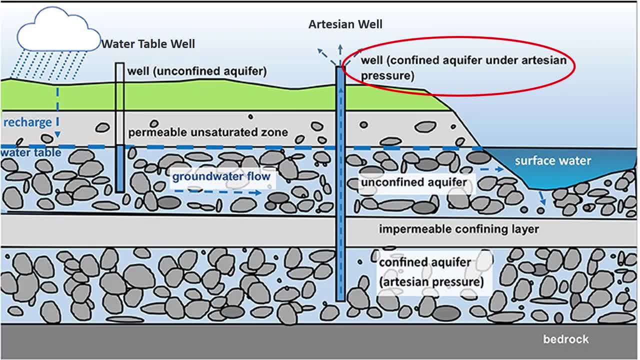 An aquifer contains saturated material that yields significant quantities of water to wells and springs. An aquifer formed under the ground can be unconfined or confined. When we dig a well penetrating a confined aquifer, we call it an artesian well. 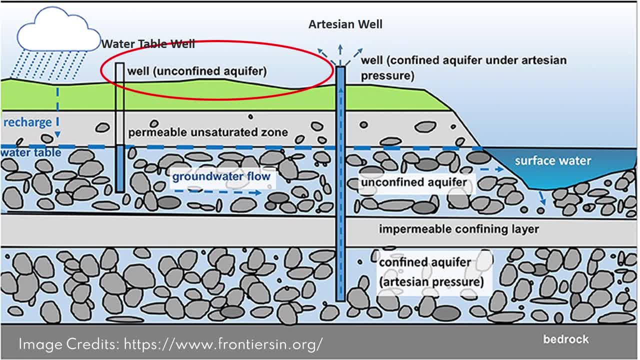 And when we dig a well penetrating an unconfined aquifer, then it is called a water table. well, As aquifer is the major source of water, it forms a major study of groundwater hydrology. More on aquifers and their types will be provided in the upcoming videos. 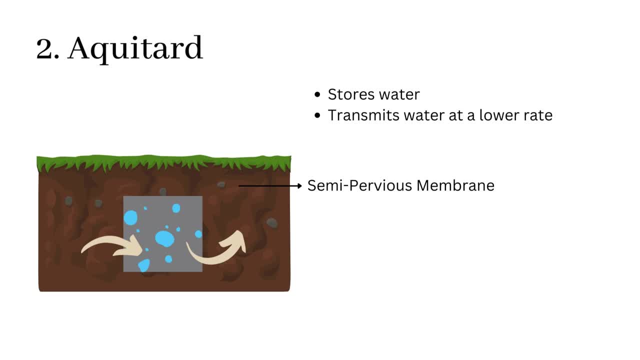 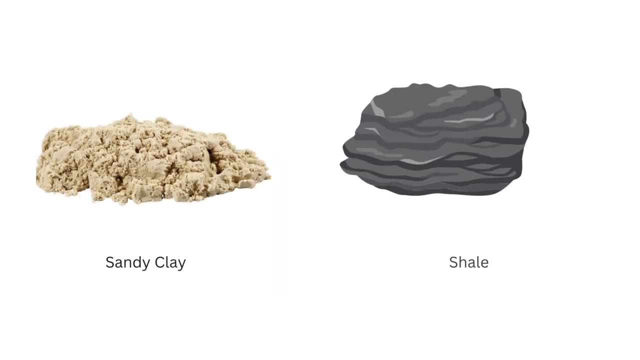 Two aquitard. An aquitard is a geological formation with a poorly permeable or semipervious membrane that only permits the storage of water, but are not capable of transmitting water in sufficient quantity. Sandy clay, shell and silty clays are examples of such formations.